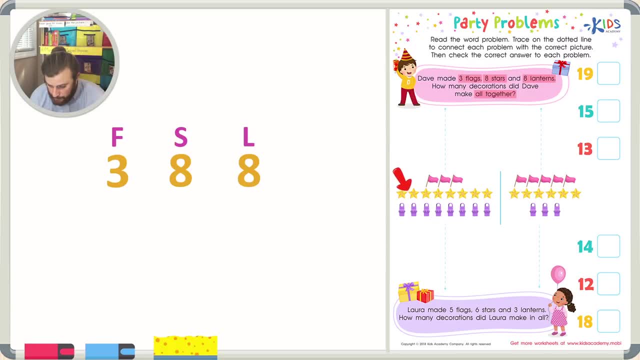 I know there's eight stars, so let's count the stars One, two, three, four, five, six, seven, eight. I also know there's eight lanterns, so let's count the lanterns: One, two, three, four, five, six, seven, eight. 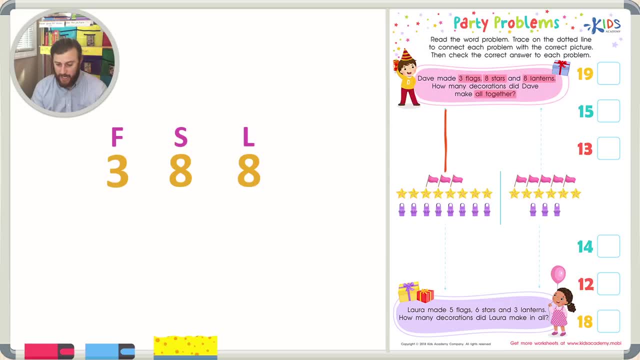 So this must be the correct equation. So let's trace on the dotted line. The question asks: how many decorations did Dave make all together? So we're going to have to add three plus eight plus eight to find out how many decorations Dave made in total, or all together. 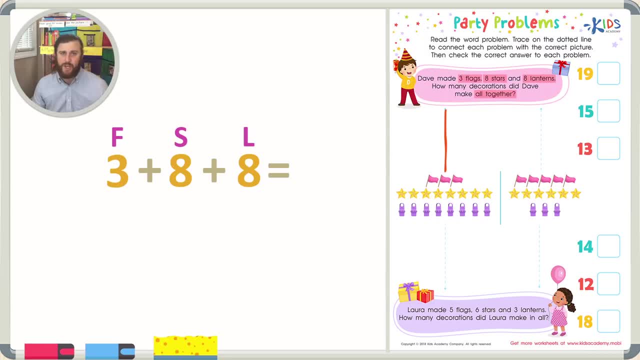 So we can add in any order that we want, because the commutative property says so. So let's add the doubles fact of eight plus eight. I know that eight plus eight is sixteen. That's one of my doubles facts. We can bring down what we have left over, which is three plus 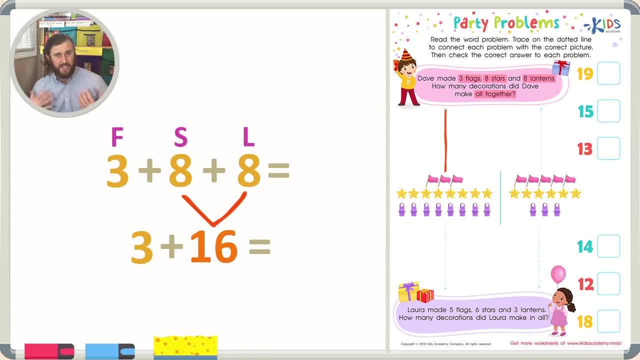 which makes our new problem three plus sixteen. Let's count on three from sixteen, Sixteen, seventeen, eighteen, nineteen. So three plus sixteen is nineteen. So the total number of decorations that Dave made is nineteen. Let's read our next word problem. 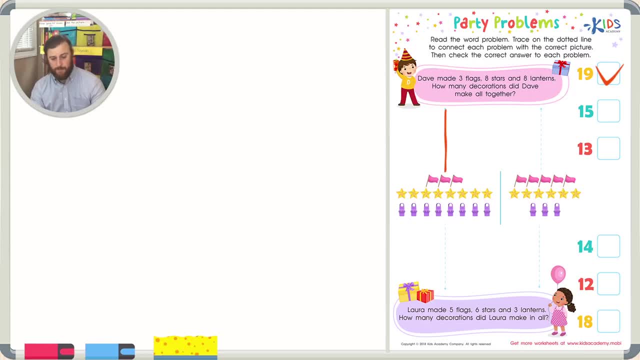 and see if we can match it to a picture to help us solve it correctly. The second problem reads: Laura made five flags, six stars and three lanterns. How many decorations did Laura make in all? Okay, let's reread this problem and again we'll underline the important information in key words. 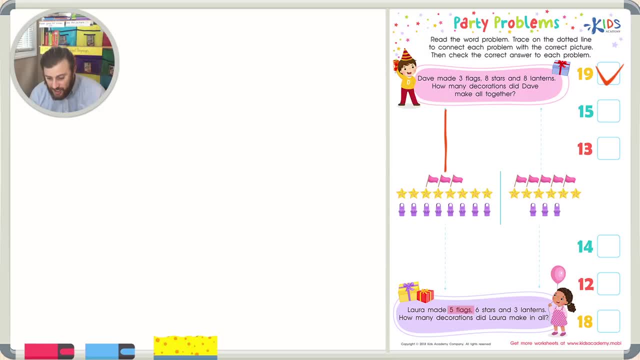 Laura made five flags, six stars and three lanterns. How many decorations did Laura make in all? Okay, so I hear that key word in all. So again, I think we're going to be adding everything up together to find out how many we have in all. 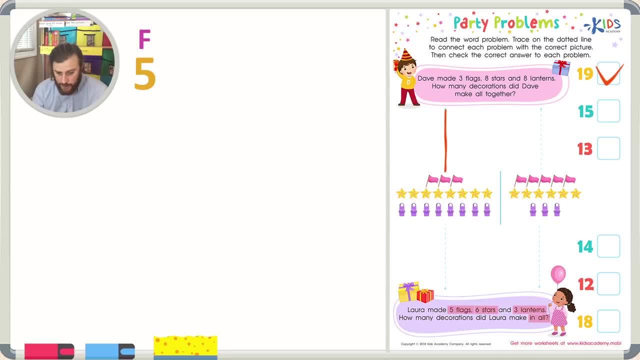 I know she made five flags, six stars and three lanterns. So let's look at the picture to see which one shows five flags, six stars and three lanterns. Well, in this picture I see one, two, three, four, five flags. so I think that's correct. 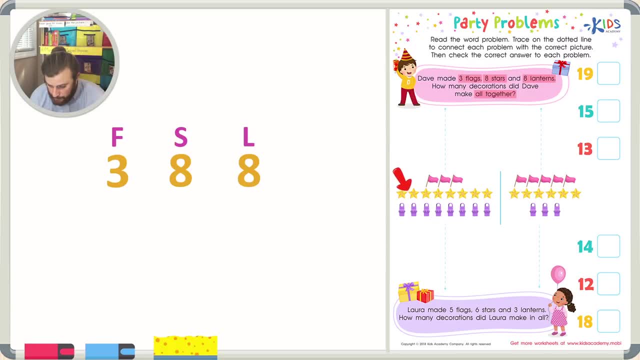 I know there's eight stars, so let's count the stars One, two, three, four, five, six, seven, eight. I also know there's eight lanterns, so let's count the lanterns: One, two, three, four, five, six, seven, eight. 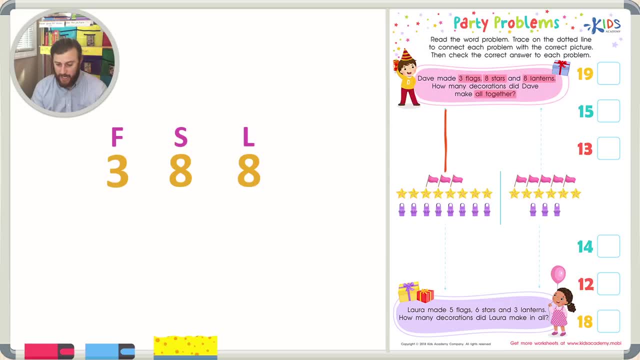 So this must be the correct equation. So let's trace on the dotted line. The question asks: how many decorations did Dave make all together? So we're going to have to add three plus eight plus eight to find out how many decorations Dave made in total, or all together. 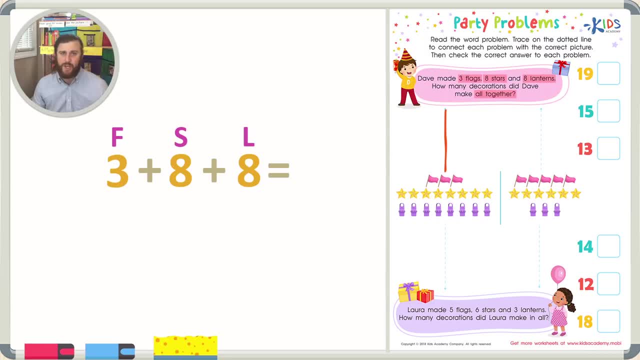 So we can add in any order that we want, because the commutative property says so. So let's add the doubles fact of eight plus eight. I know that eight plus eight is sixteen. That's one of my doubles facts. We can bring down what we have left over, which is three plus 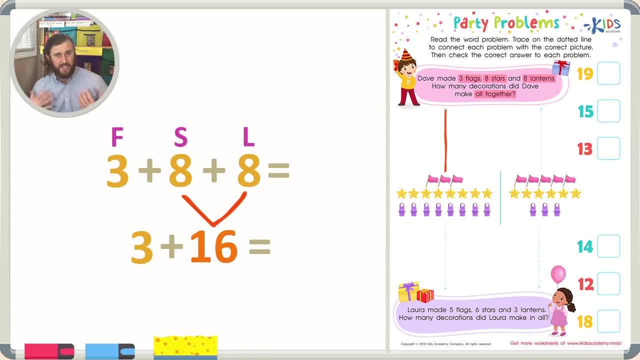 which makes our new problem three plus sixteen. Let's count on three from sixteen, Sixteen, seventeen, eighteen, nineteen. So three plus sixteen is nineteen. So the total number of decorations that Dave made is nineteen. Let's read our next word problem. 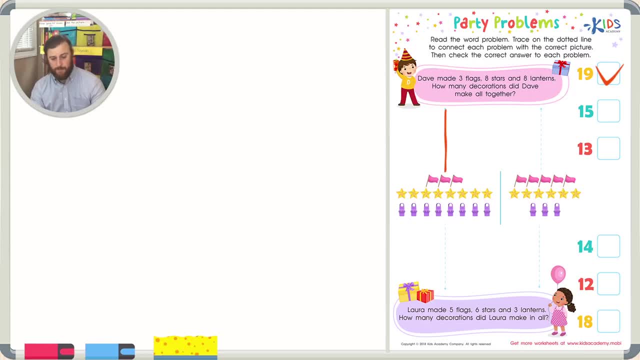 and see if we can match it to a picture to help us solve it correctly. The second problem reads: Laura made five flags, six stars and three lanterns. How many decorations did Laura make in all? Okay, let's reread this problem and again we'll underline the important information in key words. 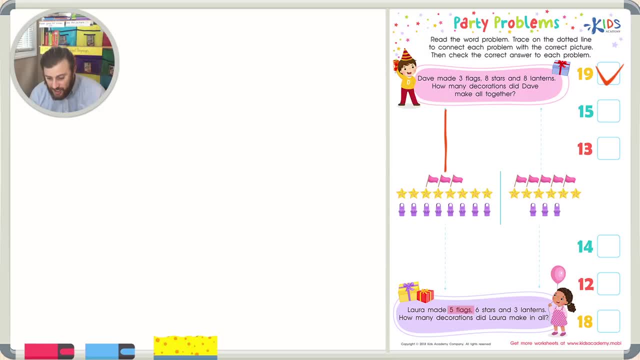 Laura made five flags, six stars and three lanterns. How many decorations did Laura make in all? Okay, so I hear that key word in all. So again, I think we're going to be adding everything up together to find out how many we have in all. 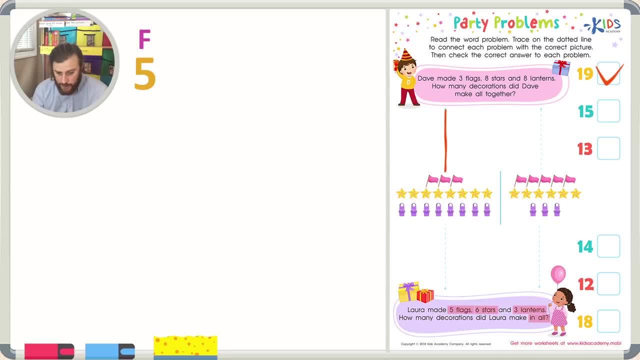 I know she made five flags, six stars and three lanterns. So let's look at the picture to see which one shows five flags, six stars and three lanterns. Well, in this picture I see one, two, three, four, five flags. so I think that's correct.